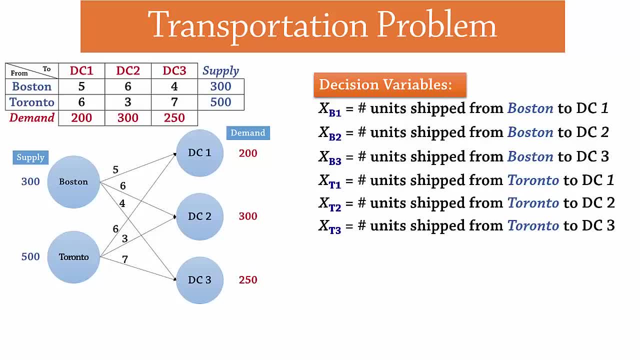 The number of decision variables is simply the number of origins multiplied by the number of destinations, In this case 2 times 3, which equals 6 decision variables. Now suppose I don't like listing every single variable, or maybe I just happen to have too. 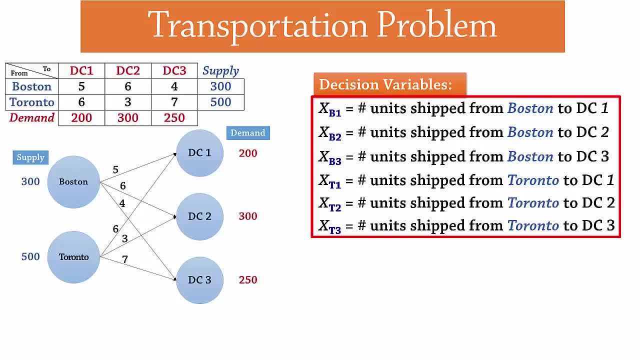 many variables, Then I can use the short form as follows: Let XIJ equal the number of units shipped from Plant I to DCJ, where I equals B for Boston and T for Toronto and J equals 123 for DC1,, DC2, and DC3 respectively. 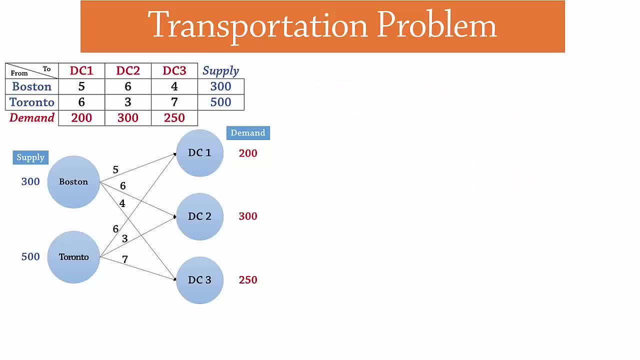 Next we can state the objective function. Since the objective function is to minimize cost, we write the objective function as follows: Minimize 5 times the number of units shipped from Boston to DC1.. Plus 6 times the number of units shipped to DC2, and so on. 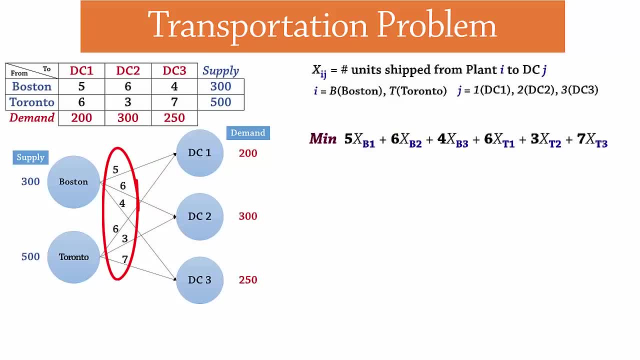 Note that every single cost is accounted for in the objective function. For the constraints, we need to write 1 for every node For Boston's supply. the total amount shipped to the 3 destination centers cannot exceed Boston's capacity, which is 300. 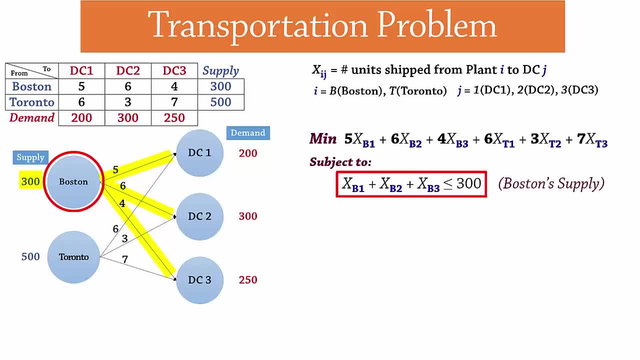 So we write: XB1 plus XB2 plus XB3 is less or equal to 300.. We do the same for Toronto: XT1 plus XT2 plus XT3 is less than or equal to 500.. Note here that total supply exceeds total demand. 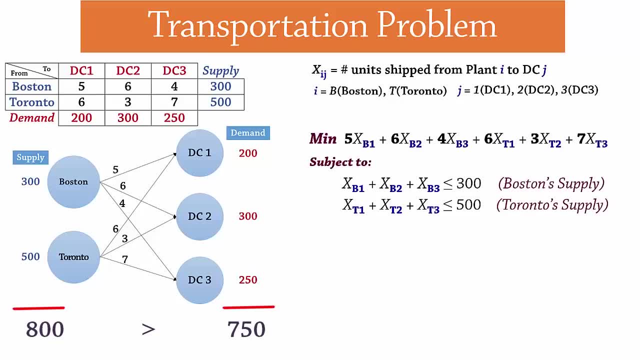 That is, we will not end up exhausting capacity, And that's why we use the less than or equal sign For DC1 node. we write: XB1 plus XT1 equals 200.. Equality is used because we have a demand here that must be met and we have enough. 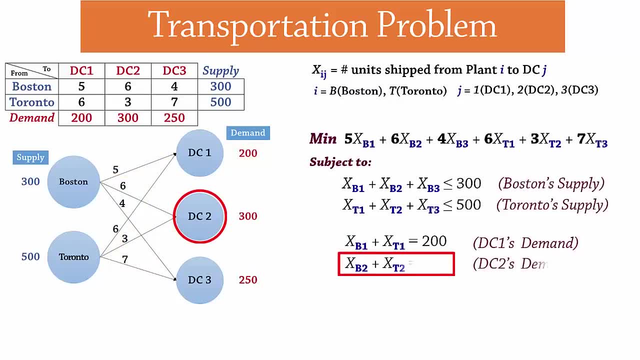 supply to meet it. Similarly, for DC2, we have: XB2 plus XT2 equals 300.. And for DC3, we have: XB3 plus XT3 equals 250.. For non-negativity, we can either list all the variables and state that each is greater. 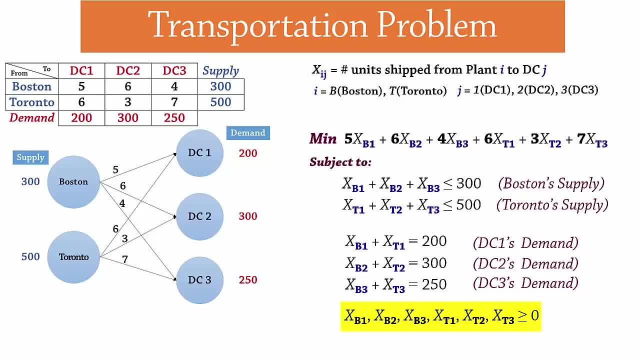 than or equal to 0.. Or we can simply write: Xij is greater or equal to 0, for all i and j, And that's the LP model. Furthermore, let's suppose the cost of producing a unit of the product is less than or equal. 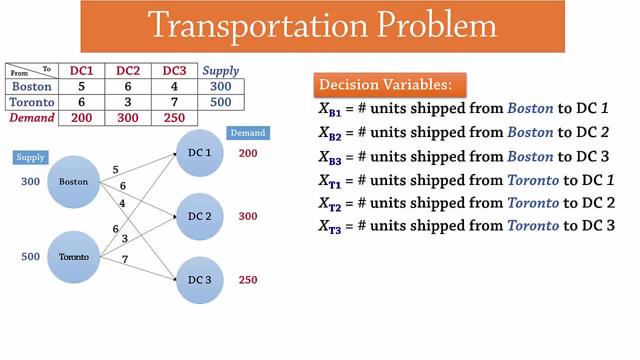 the number of origins multiplied by the number of destinations, In this case 2 times 3, which equals 6 decision variables. Now suppose I don't like listing every single variable, or maybe I just happen to have too many variables. Then I can use the. 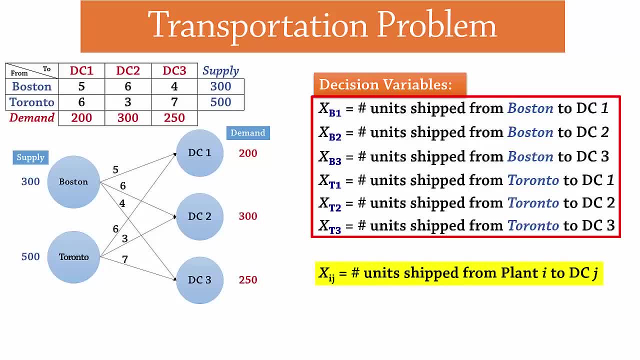 short form as follows: Let Xij equal the number of units shipped from plant i to DCj, where i equals B for Boston and T for Toronto and j equals 123 for DC1, DC2 and DC3 respectively. Next we can: 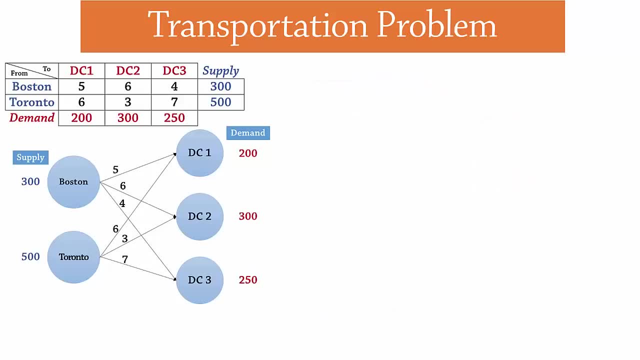 state the objective function. Since the objective function is to minimize cost, we write the objective function as follows: Minimize 5 times the number of units shipped from Boston to DC1, plus 6 units to DC1.. Minimize 5 times the number of units shipped from Boston to DC1, plus 6 units. 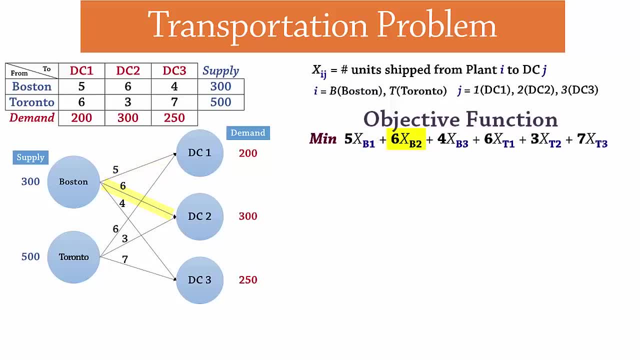 6 times the number of units shipped to DC2 and so on. Note that every single cost is accounted for in the objective function. For the constraints we need to write 1 for every node. For Boston's supply, the total amount shipped to the 3 destination centers cannot exceed Boston's. 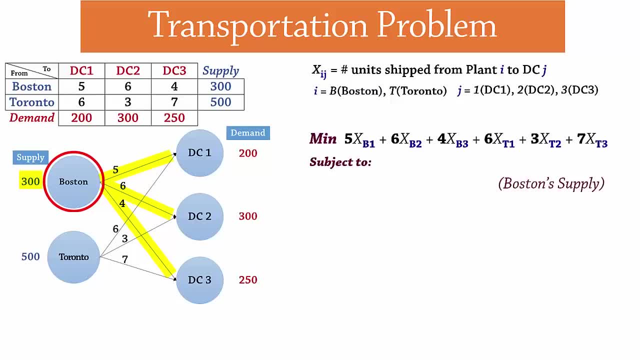 capacity, which is 300.. So we write: XB1 plus XB2 plus XB3 is less or equal to 300.. We do the same for Toronto: XT1 plus XT2 plus XT3 is less than or equal to 500.. Note here that total supply exceeds total demand, That is, we will not end up exhausting capacity. 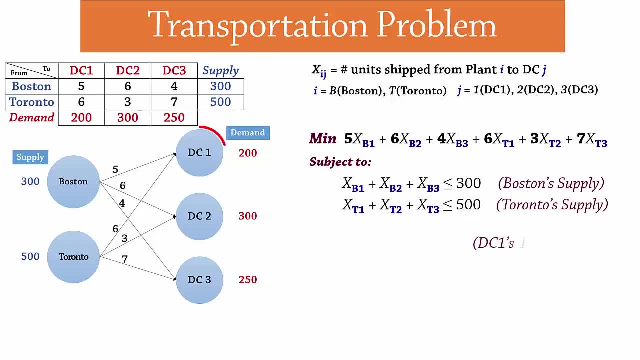 And that's why we use the less than or equal sign. For DC1 node we write: XB1 plus XT1 equals 200.. Equality is used because we have a demand here that must be met and we have enough supply to meet it. 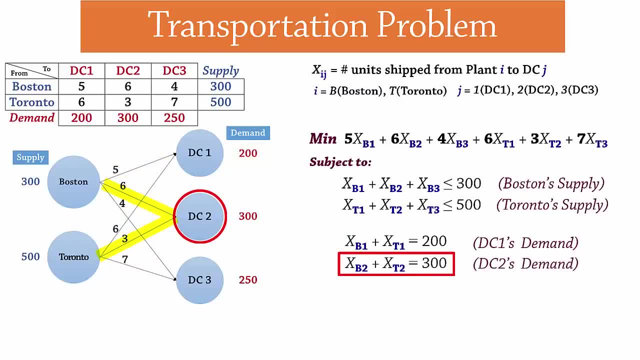 Similarly, for DC2, we have, XB2 plus XT2 equals 300, and for DC3, we have, XB3 plus XT3 equals 250.. For non-negativity, we can either list all the variables and state that each is greater than. 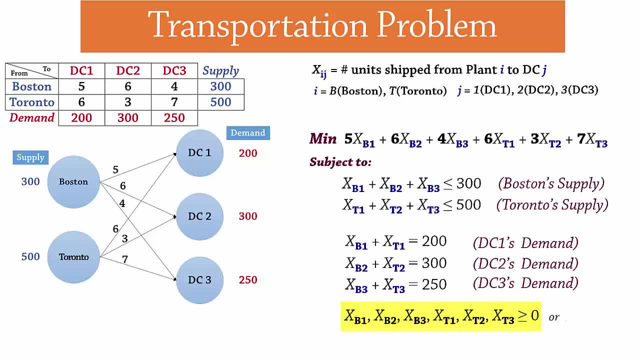 or equal to 0, or we can simply write: Xij is greater or equal to 0 for all i and j, And that's the LP model. Furthermore, let's suppose the cost of producing a unit of the product is $20 in Boston and $18 in Toronto. Then we simply add $20 to the shipping cost per unit. 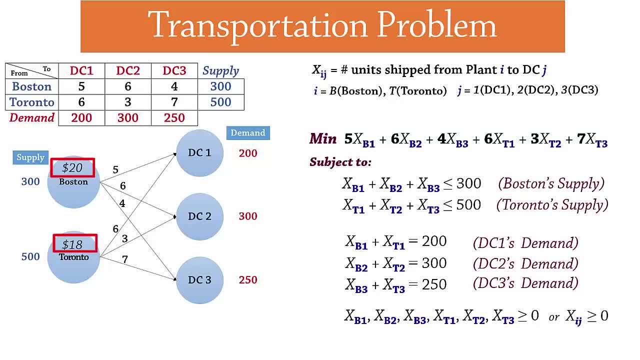 to $20 in Boston and less than $18 in Toronto, Then we simply add 20 to the shipping cost per unit of the product from Boston and add 18 to those from Toronto. The objective function is thus updated accordingly. Note here that if total supply were to equal total demand, we could have used equality. 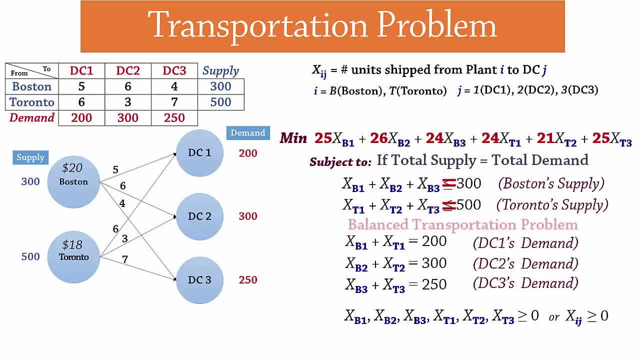 for all constraints. We refer to that situation as a balanced transportation problem. This problem, however, is an unbalanced transportation problem. It is a problem that requires a balanced transportation system. This is a balanced transportation example where supply exceeds demand. Moreover, we could also have an unbalanced problem where demand exceeds supply. 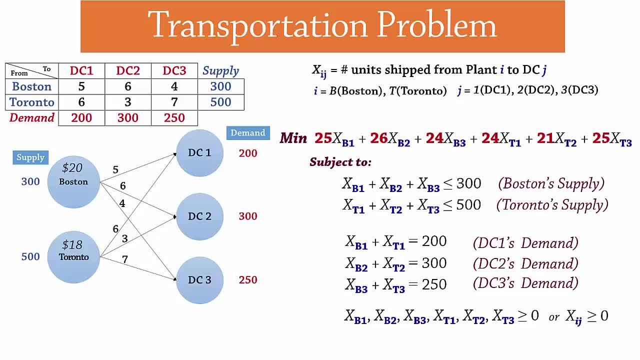 Consider the following scenario. Suppose demand at DC1 increases to 300 units, Then we have another unbalanced problem with demand exceeding supply. Let's look at two ways to handle this, Since demand now exceeds supply by 50 units, one approach is to add a dummy plant and assign. 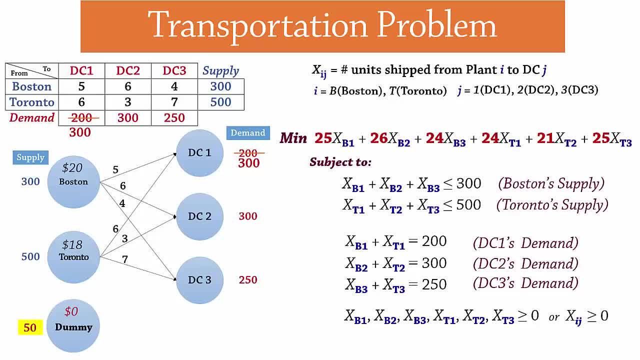 it a supply of 50 units. Note that these 50 units do not exist, So their cost per unit is zero and their shipping cost is also zero, since they are not going to be shipped at all. We can thus modify our model as follows: 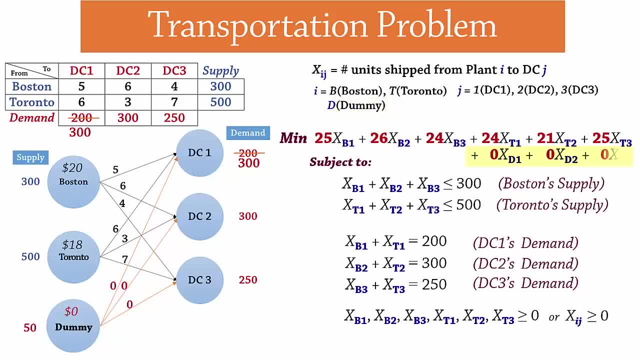 Add D for dummy in the decision variables. Add the new cost to the objective function. They won't really have an impact on total cost. Next, we add a constraint for the dummy node And then add the units assumed to be shipped from the dummy to the distribution system. 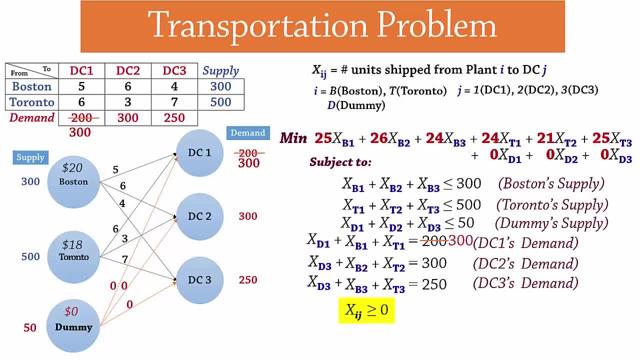 Add the units assumed to be shipped from the dummy to the distribution center And again, xij is non-negative for all i and j. At the end of the day, demand will not be fully satisfied at some of the distribution centers because the dummy supplies don't really exist. 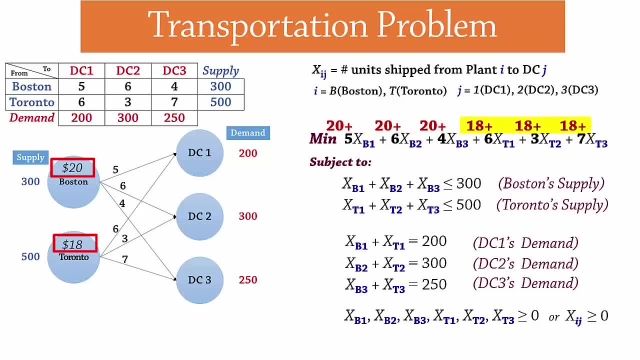 of the product from Boston and add $18 to those from Toronto. The objective function is thus updated accordingly. Note here that if total supply were to equal total demand, we could have used equality for all constraints. We refer to that situation as a balanced transportation problem. This problem, however, is an unbalanced transportation. 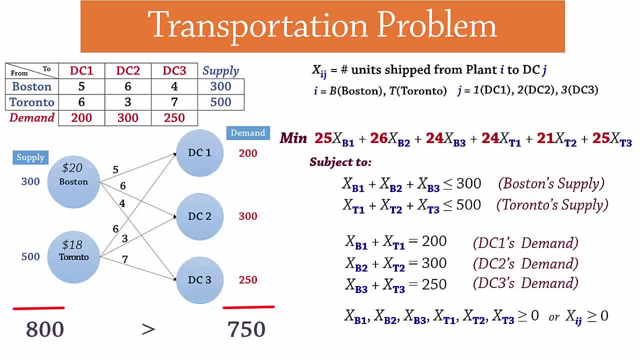 example, where supply exceeds demand. Moreover, we could also have an unbalanced problem where demand exceeds supply. Consider the following scenario: Suppose demand at distribution center 1 increases to 300 units, Then we have another unbalanced problem with demand exceeding supply. Let's look at two ways to handle this, Since 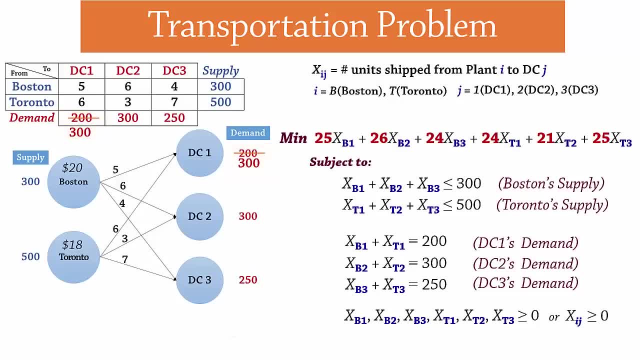 demand now exceeds supply by 50 units. one approach is to add a dummy plant and assign it a supply of 50 units. Note that these 50 units do not exist, so their cost per unit is zero and their shipping cost is also zero, since they are not going to be shipped at. 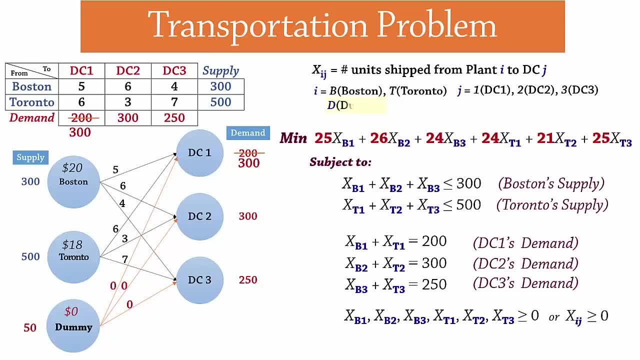 all. We can thus modify our model as follows: Add d for dummy in the decision variables. Add the new cost to the objective function. They won't really have an impact on total cost. Next we add a constraint for the dummy node And then add the units assumed to be shipped. 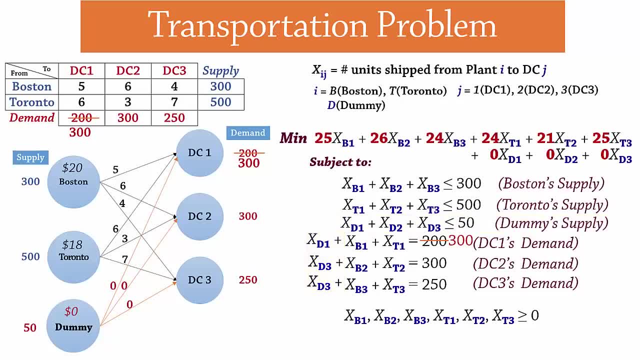 from the dummy to the distribution center. And again, Xij is non-negative for All i and j. At the end of the day, demand will not be fully satisfied at some of the distribution centers because the dummy supplies don't really exist. 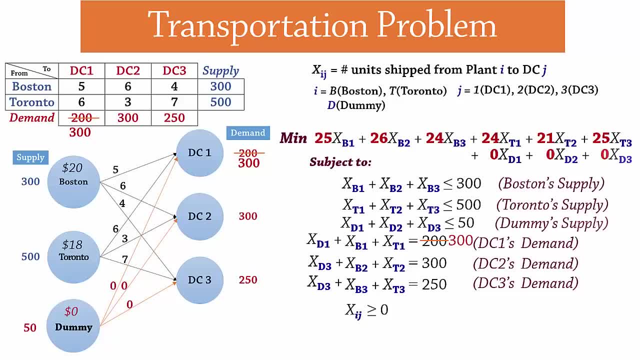 Instead of introducing a dummy, let's now look at another formulation method we could apply. Since demand exceeds supply, all available supply will be used-up, so we simply change the less than or equal signs here to equal signs. Since demand is not going to be fully met at some of the distribution centers, we change 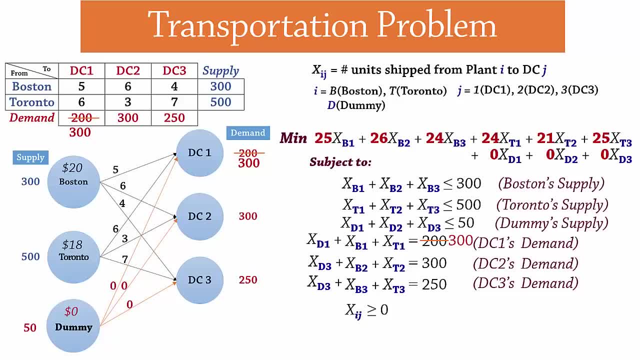 Instead of introducing a dummy, let's now look at another formulation method we could apply. Since demand exceeds supply, all available supply will be used up, So we simply change the less than or equal signs here to equal signs. And since demand is not going to be fully met at some of the distribution centers, 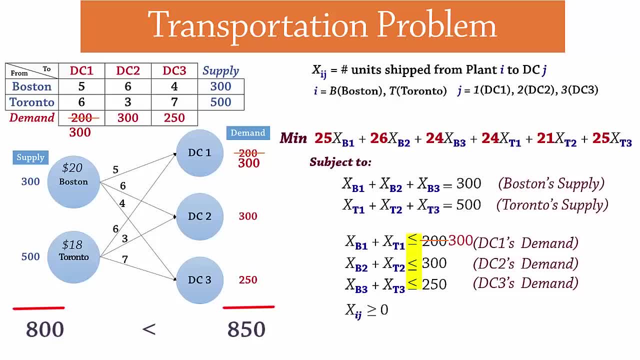 the demand equality signs to less than or equal signs, And the model is again complete. Now suppose for some reason we are not allowed to ship from Toronto to distribution center 3. Maybe because the cost is too high or the destination is too far?